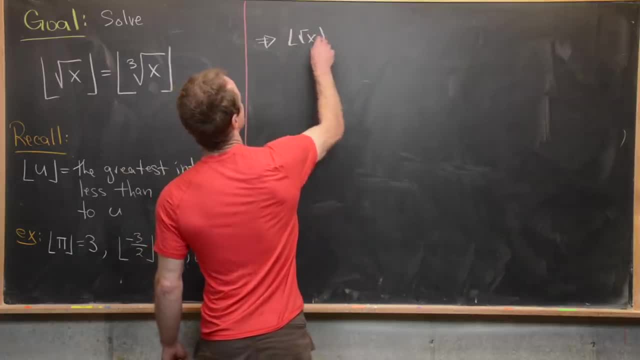 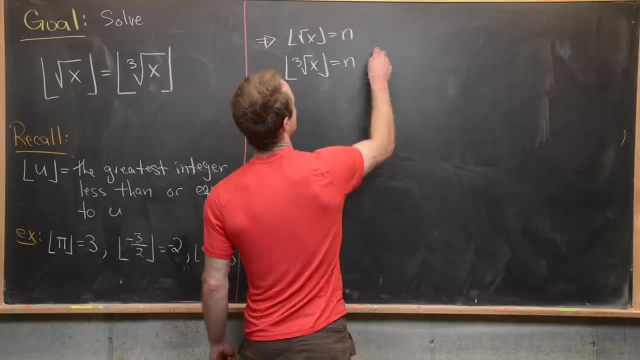 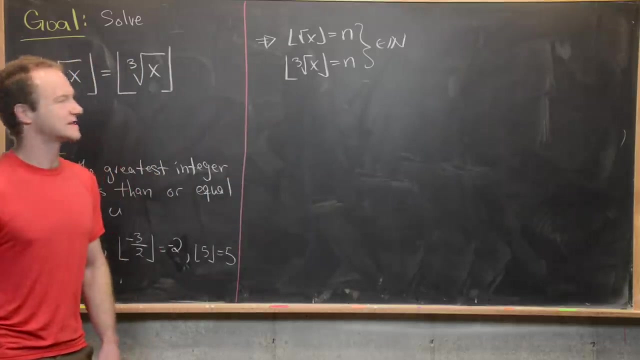 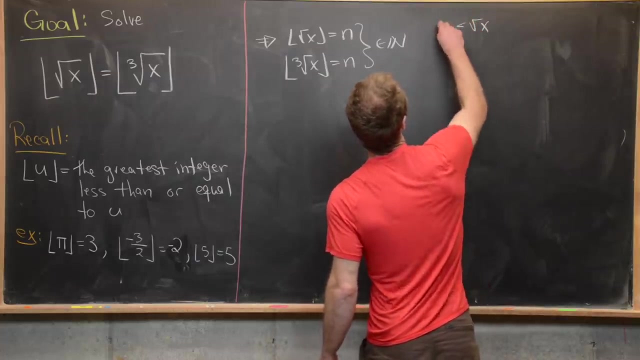 the square root of x equals n and the floor of the cube root of x equals n, where this n is the same natural number. Let's flesh out what that really means. So the floor of the square root of x being equal to n, that tells us that the square root of x is going to be bigger than or equal to, 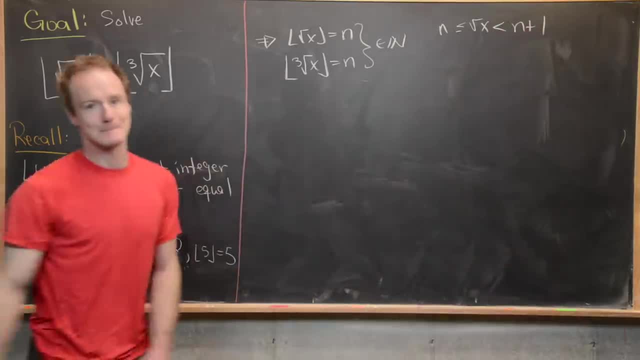 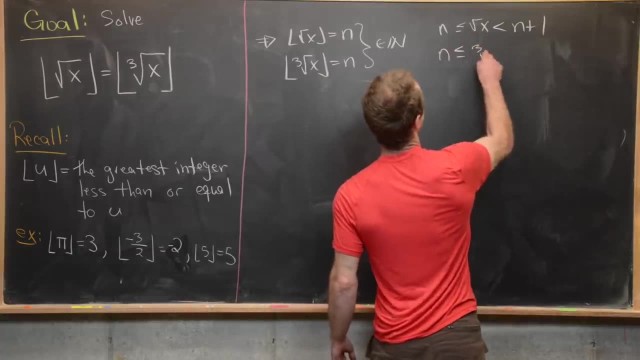 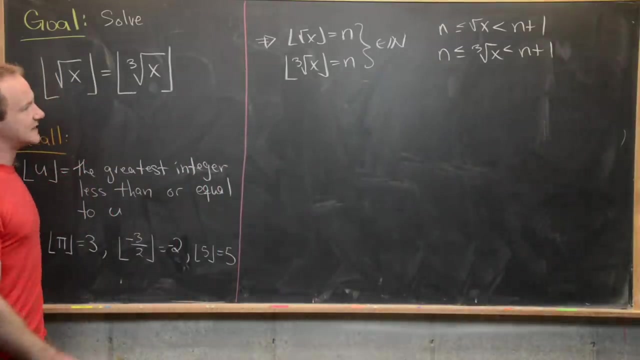 n, but strictly less than n plus 1.. And then the floor of the cube root of x being equal to n means the same kind of statement, but with the cube root of x. So we know that the cube root of x is between n and n plus 1, where n is. 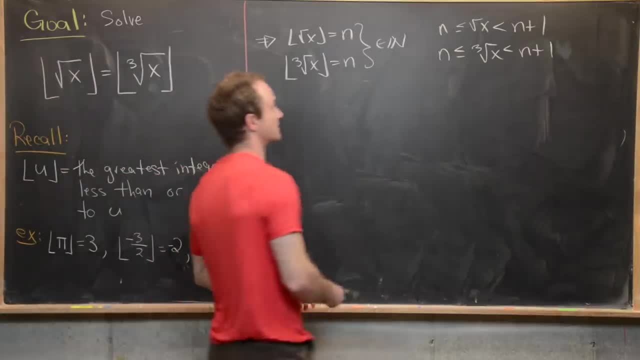 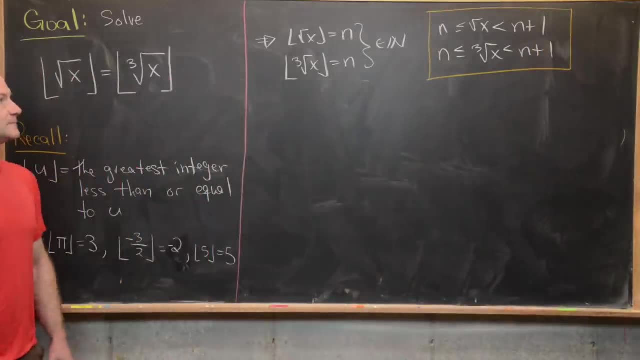 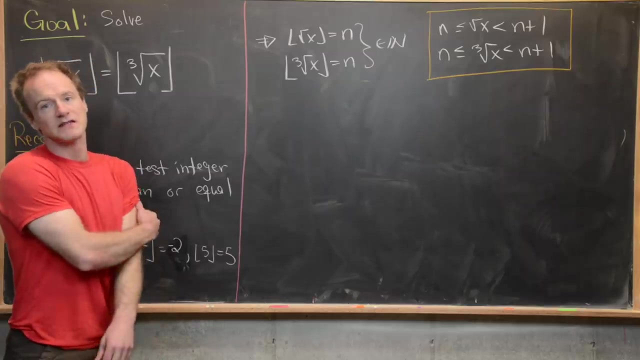 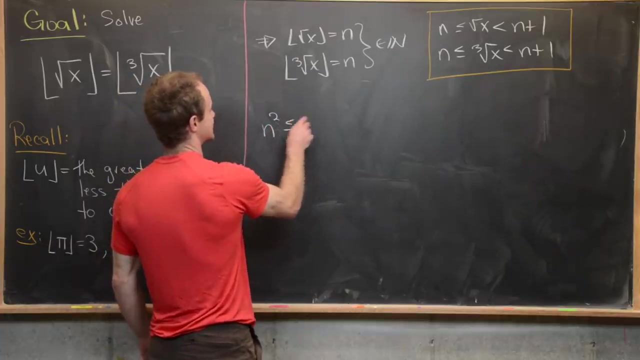 like this natural number or maybe this positive integer, really here. Okay, so we have this condition on our number x at this point. Now, next, what I want to do is maybe square the first inequality and cube the second inequality To give us an inequality involving x. so that's going to give us n. squared is less than or equal. 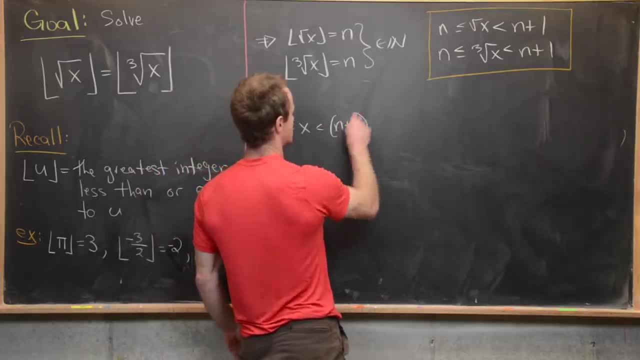 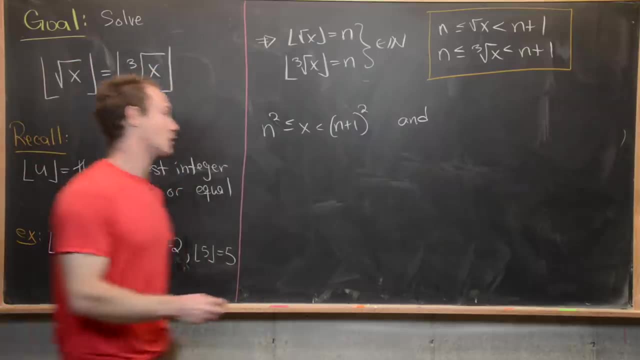 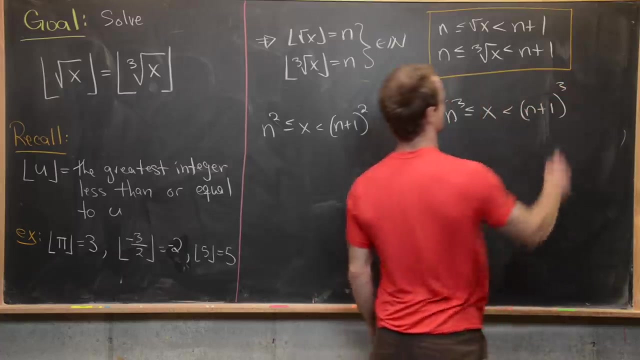 to x, which is less than n plus 1 squared, And cubing the second inequality will give us n cubed is less than or equal to x, which is less than n plus 1 cubed. But now, since we know something about the growth of the square root of x, we're going to have to figure out how to. 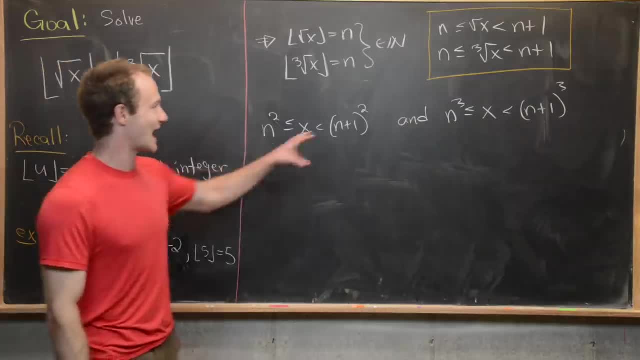 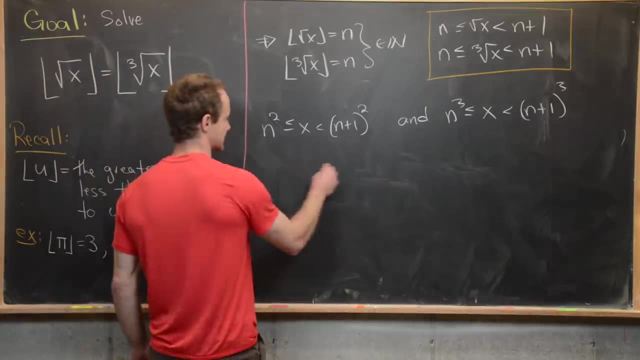 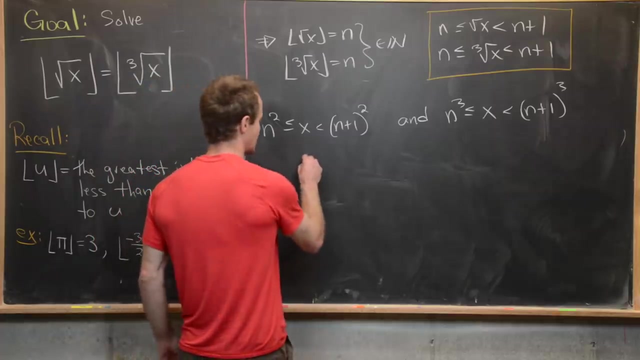 do that. So we have the squaring function versus the cubing function. We can actually mash this all together into one long inequality. That long inequality is going to go like this. So some of it is not super mind-blowing, but it is important to see kind of the structure here. So we have n. 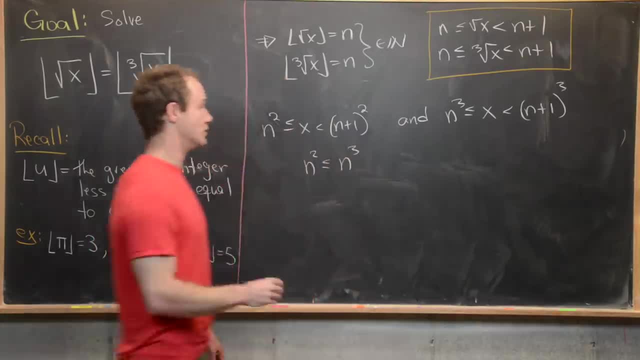 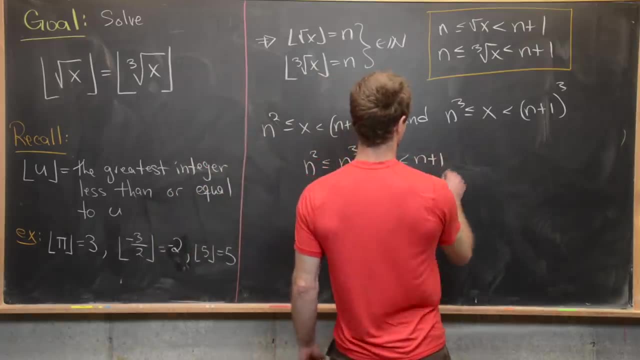 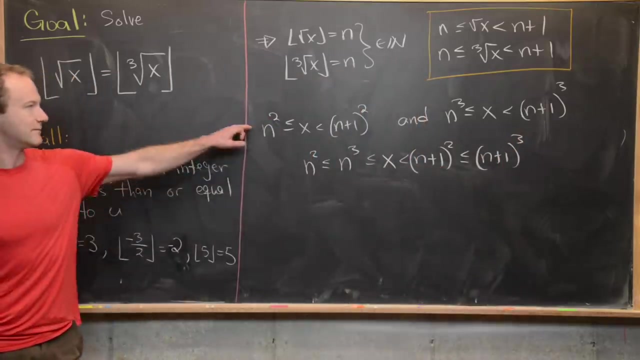 squared is less than or equal to n cubed, which is less than or equal to x, which is less than n plus 1 quantity squared. So again, mashing these two inequalities together gives us this. And now what we want to hone in on. 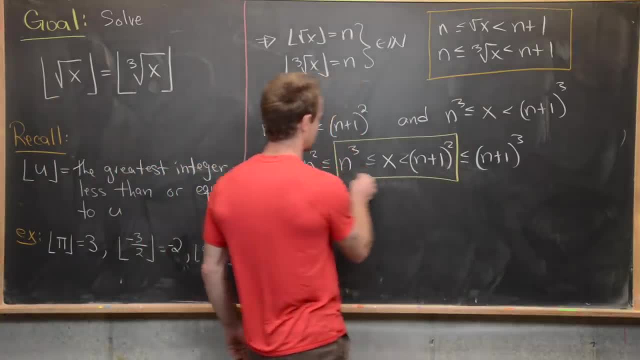 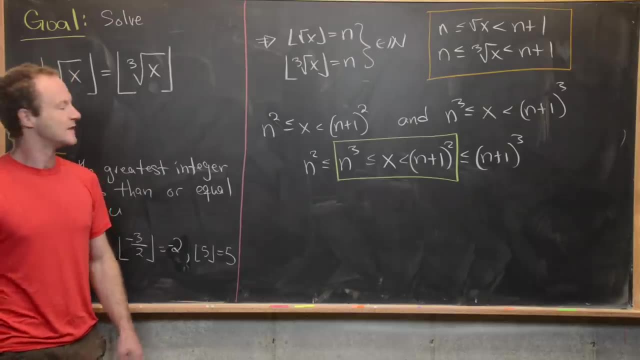 is the central inequality here: The fact that we have n cubed less than or equal to x strictly less than n plus 1 squared. And if we can find n that satisfy this inequality, then we're really in a good place. So let's maybe go ahead and do that. 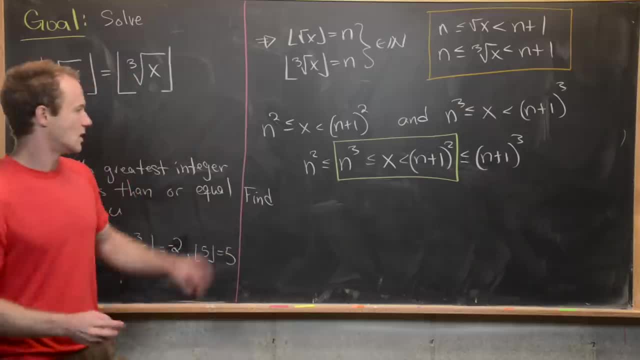 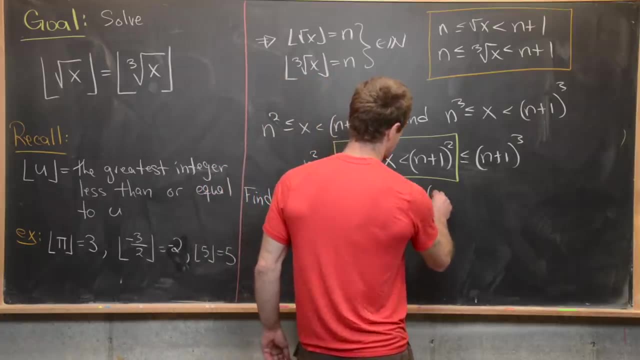 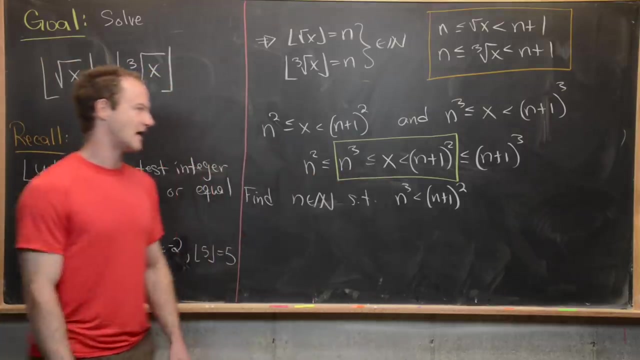 So we're going to have this kind of sub-goal which is to find n, which are natural numbers, such that n cubed is less than n plus 1 squared. Then if we can find natural numbers that satisfy that, then we just look for x values that are between there, make some tests and then we're good to go. 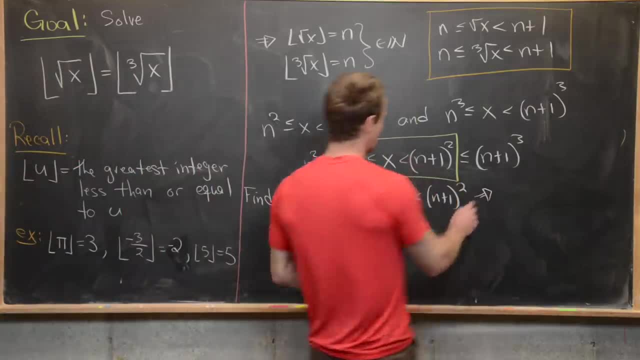 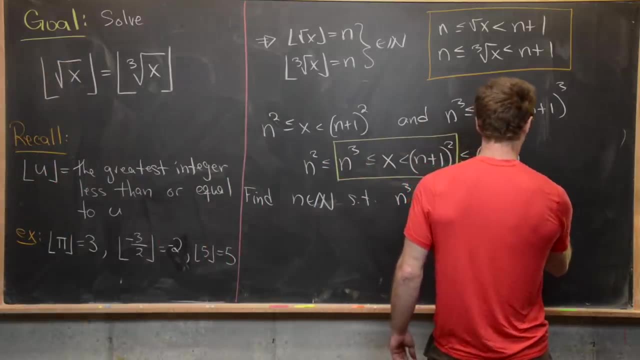 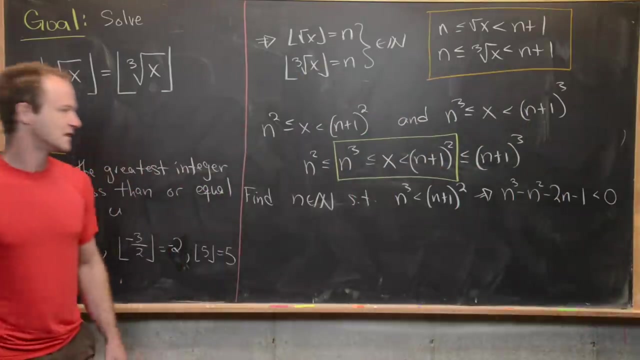 Okay, so let's maybe see how this goes, So we can change this inequality to maybe one involving zero. That'll be something like this: We'll have n cubed minus n squared minus 2n minus 1 is less than zero. 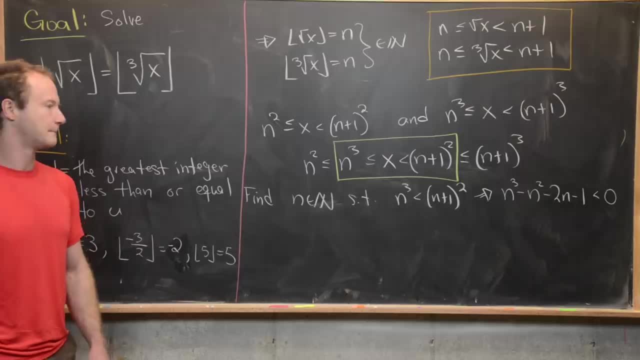 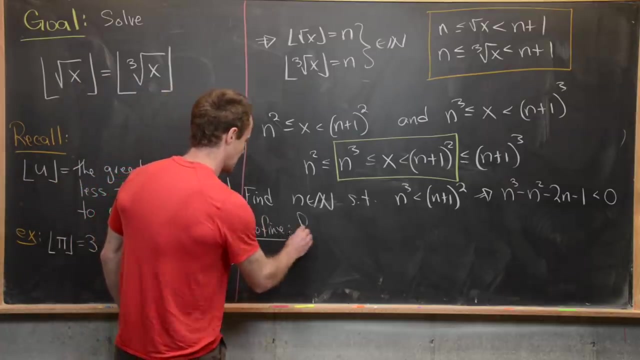 So I just squared out the right-hand side of that and moved everything over. Okay, so now we can talk about this in terms of when a function is negative at this point. So let's maybe go ahead and define this function. So I'm going to call it f and we'll have variable t. 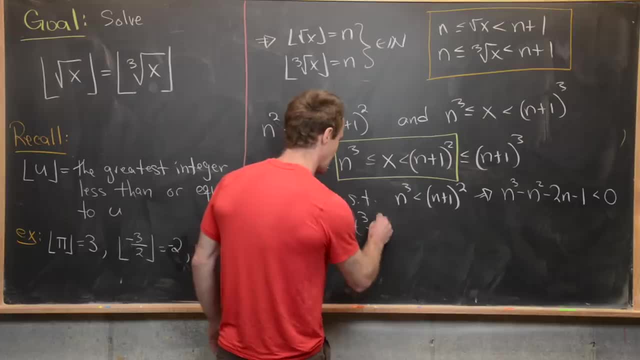 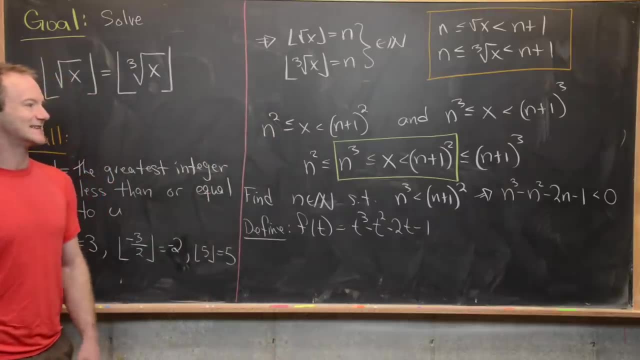 f of t is going to be equal to t cubed minus t squared minus 2t minus 1.. Now I'm not going to find exactly what the roots are of this function, because I don't really need to know that. I'm just going to find out that this function is positive after. 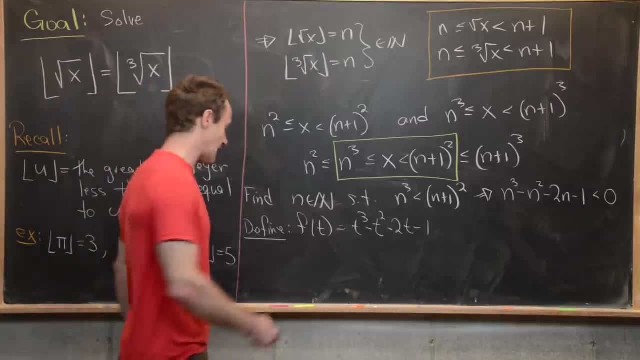 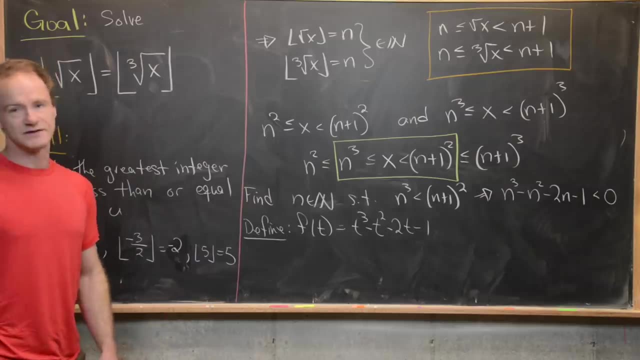 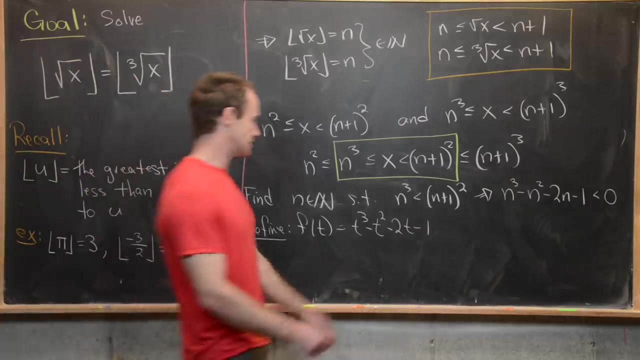 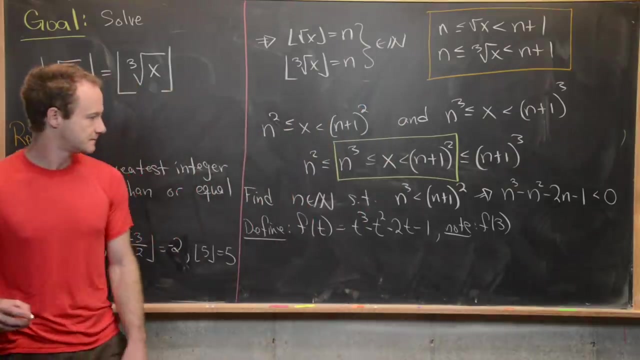 a certain point. but then, since our n value up here is either 0,, 1,, 2, so on and so forth, that restriction really gives us enough information, along with maybe knowing that this function is positive after a certain point. Good, So maybe what I first want to notice is that if I plug 3 into this function, what do I get? 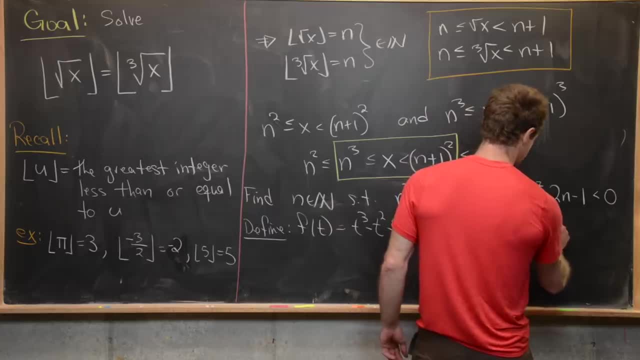 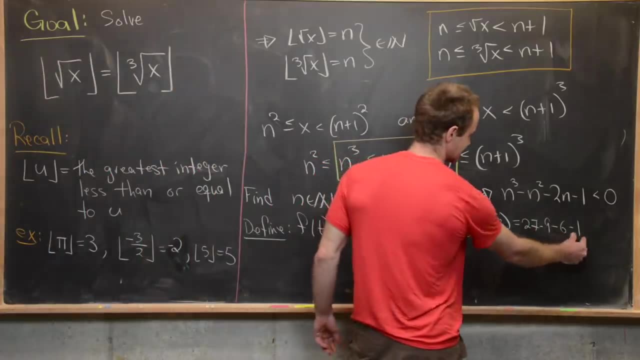 So I get 3 cubed, That's 27 minus 3. squared is 9 minus 2 times 3 is 6 minus 1.. So let's see what we get from that. So we've got 27 minus 6 minus 1 is 20 minus 9 is 11.. 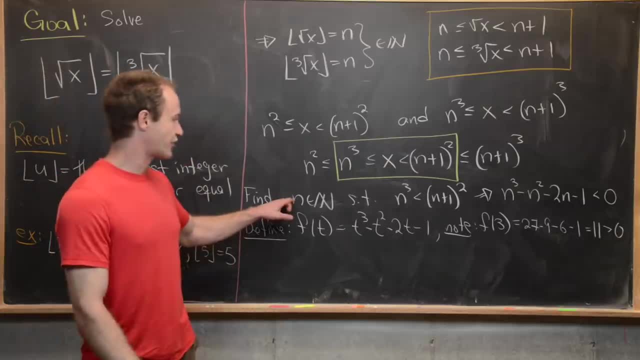 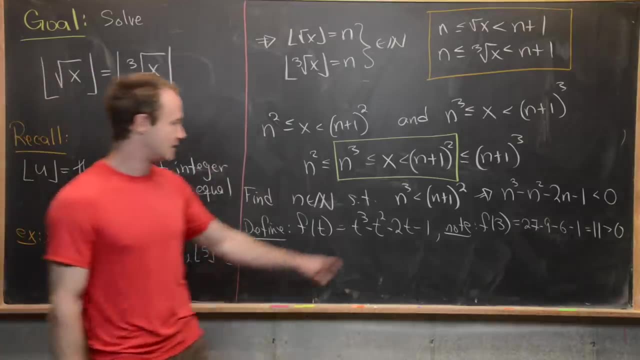 So 11 is positive. So we know that 3 is not one of the numbers that makes this inequality satisfied. And I mean we can check that by hand. Notice: 3 squared is equal to sorry, 3 cubed is equal to 27.. 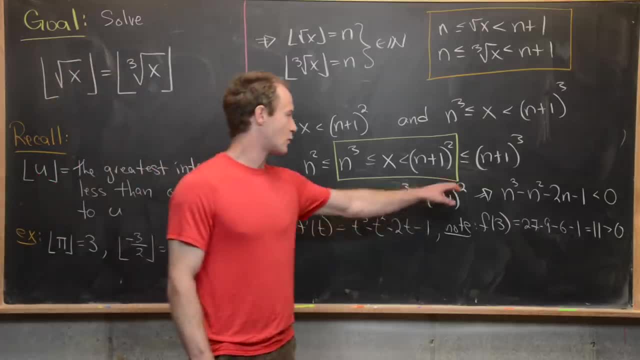 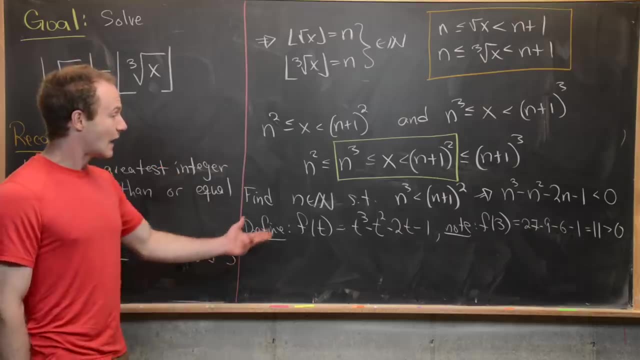 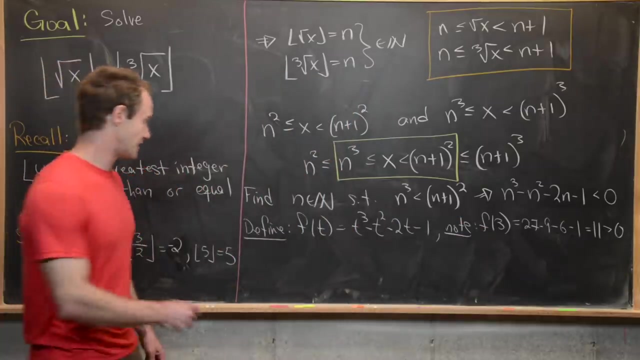 But then 3 plus 1 is 4.. 4 squared is equal to 16,, but 27 is not less than 16.. So 3 does not work here. Now what we want to show is that this function is in increasing for all t values bigger than 3.. So that's the next thing that we'll show. 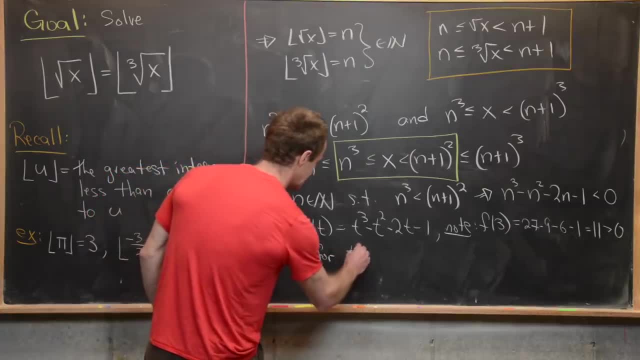 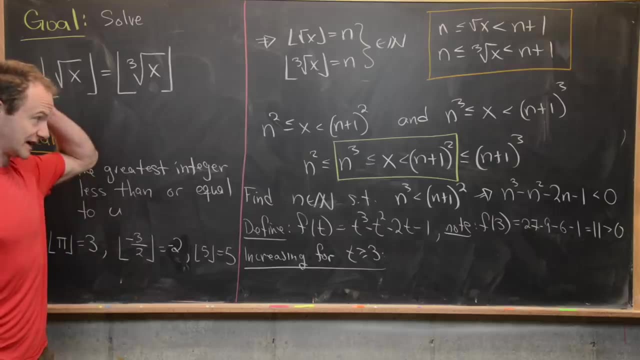 that this thing is increasing for t bigger than or equal to 3.. And we're going to do that just with the first derivative test. So, in other words, we're going to take the derivative of this function, find out where that derivative is 0,. 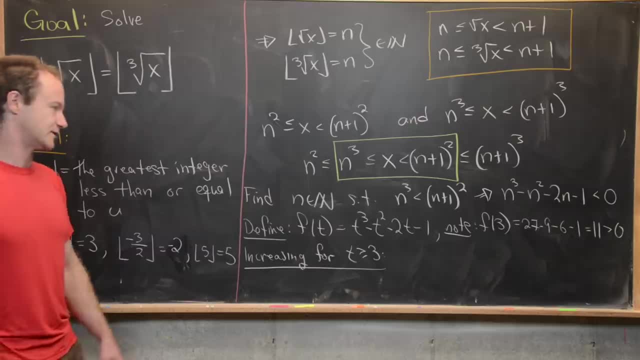 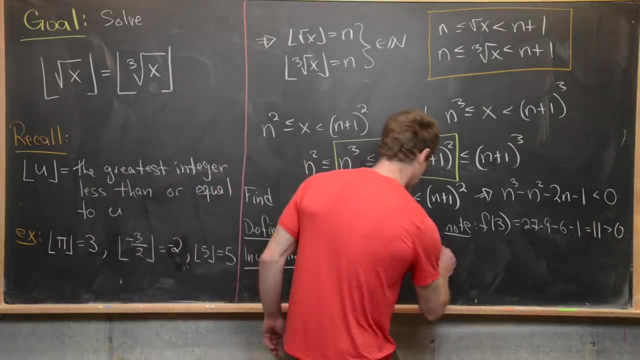 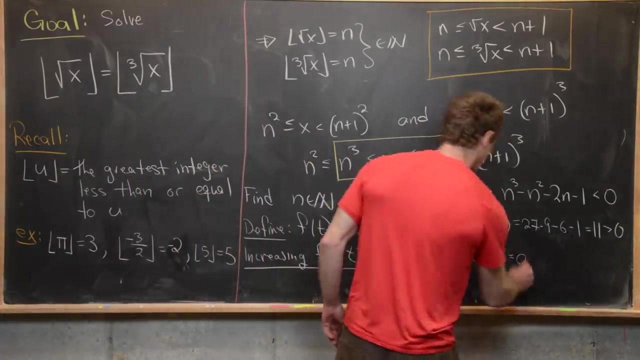 and then pick a test point to the right of that place where the derivative is 0. So maybe the derivative of this, just using the power rule, is going to be 3t squared minus 2t minus 2.. We want to set that equal to 0 to find the critical points. 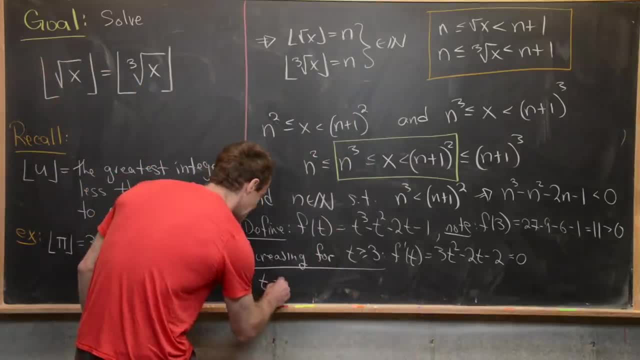 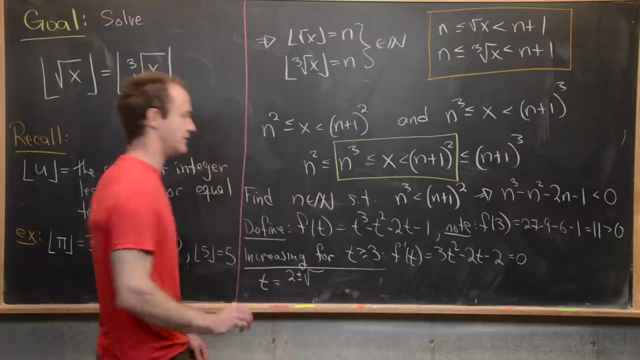 Notice. we're probably going to want to use the quadratic formula for that. We're going to get t equals, so it'll be negative b. So let's see that is going to be 2 plus minus the square root of b squared minus 4ac. 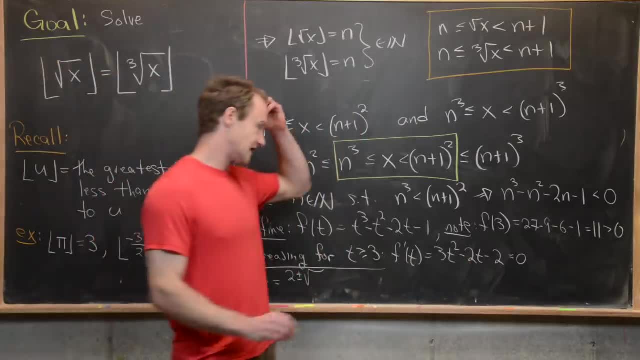 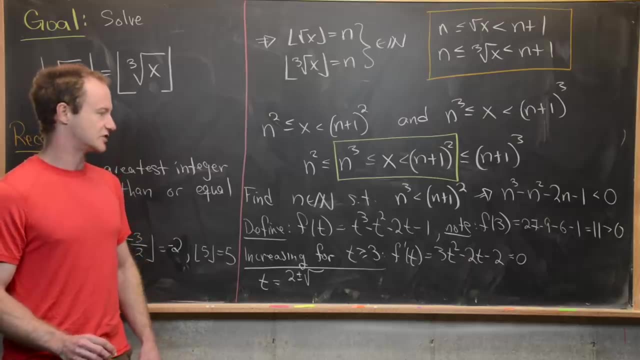 So b squared is 4 minus 4 times 2.. So that's going to be 2.. That's going to be 4 times a times c. So let's see, it's going to be 4 times 3, which is 12, times 2,, which is 24.. 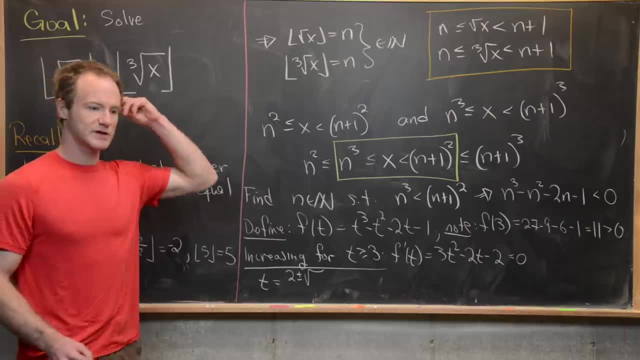 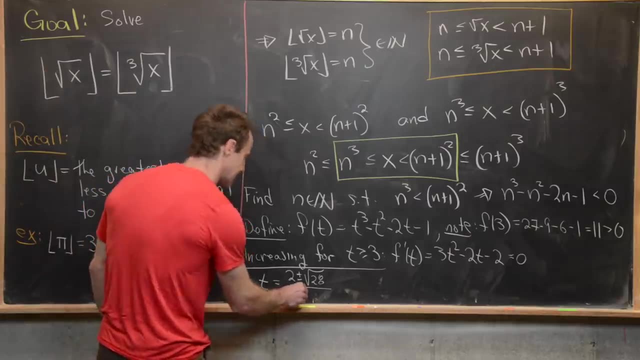 So we have 4 plus 24 there. Let's see, 4 plus 24 is going to be 28.. And that's going to be all over 2 times 8, so that's going to be all over 6.. 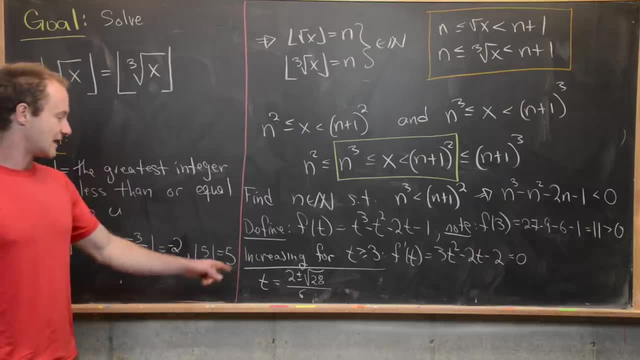 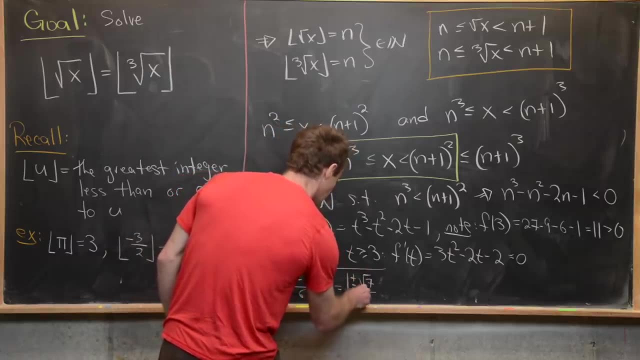 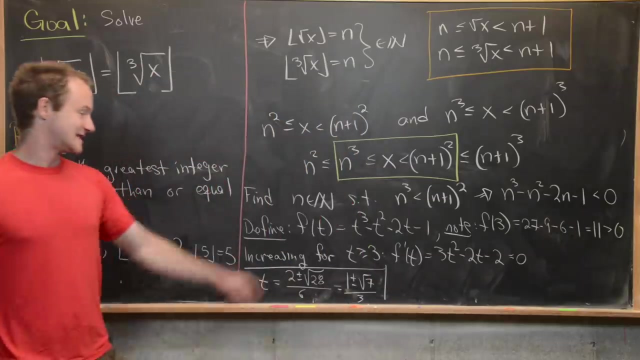 And then you guys can check maybe that that can simplify pretty easily to 1 plus or minus the square root of 6.. So that's going to be 7 over 3.. Okay, great Now. what I want to notice next is that 3 is larger than either of those roots. 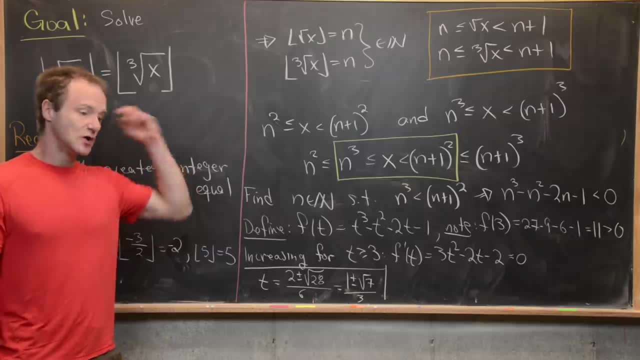 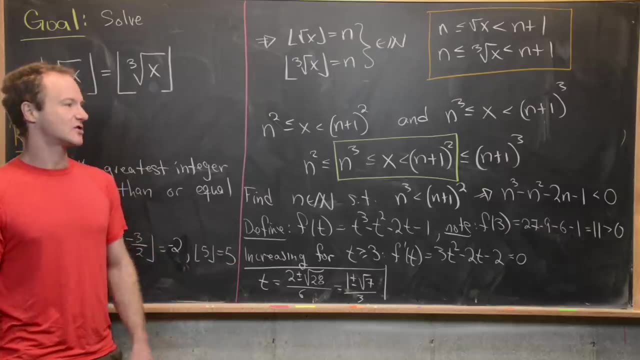 And so, since 3 is larger than either of those roots, we can use 3 as a test point. So let's just reiterate what's going on here. So the only place that this function can change from increasing to decreasing or decreasing to increasing, 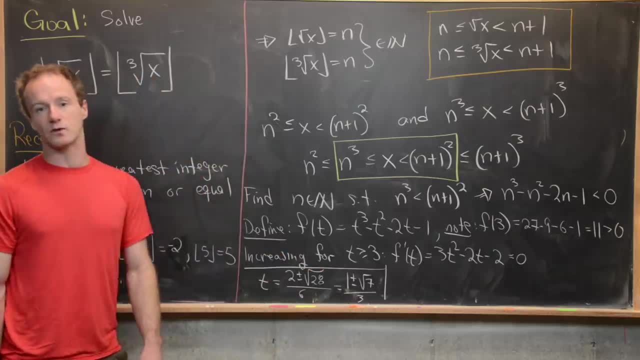 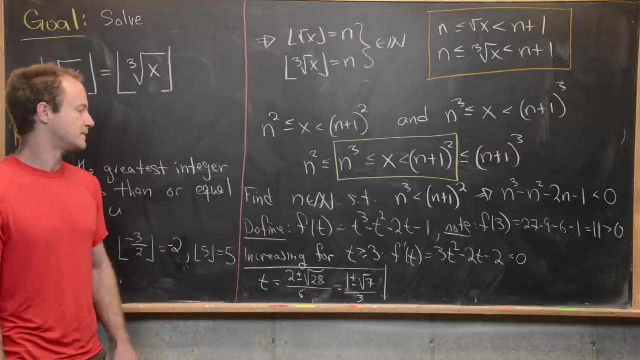 Is at these critical points, In other words when the derivative equals 0.. So the derivative equals 0 at 1 minus root 7 over 3 and 1 plus root 7 over 3.. So the number 3 is to the right of 1 plus root 7 over 3.. 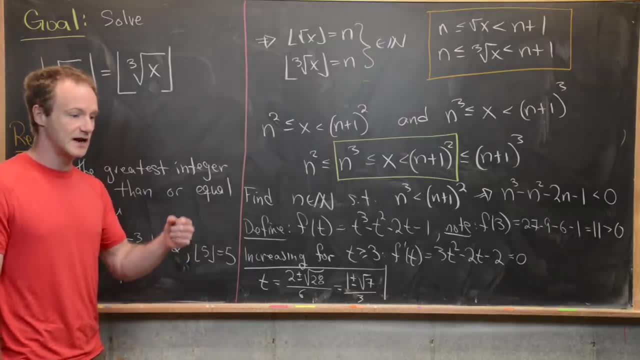 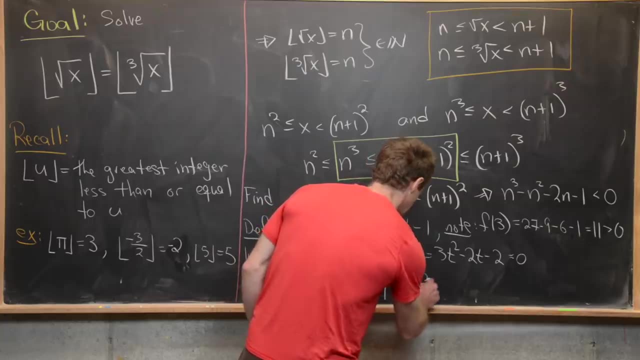 So if the function is increasing at the number 3, then it's increasing for all t bigger than 3.. So let's go ahead and check f prime of 3.. Okay, So we're going to use 3 to see what's happening at 3.. 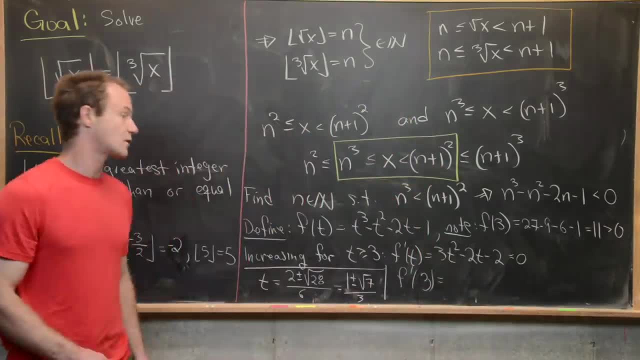 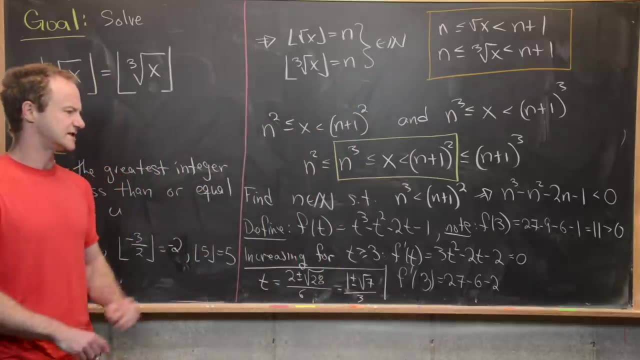 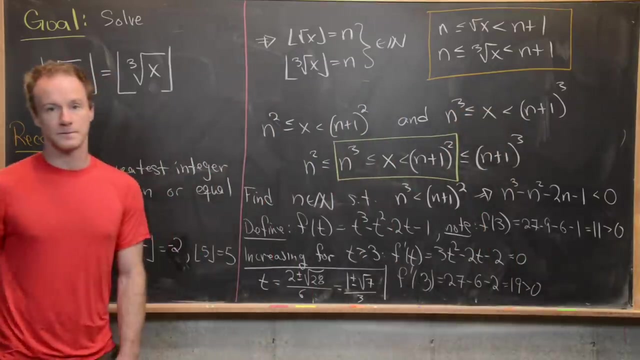 So that's going to give us 3 times 3 squared. So that's going to be 27 minus 6 minus 2.. So let's see, 27 minus 6 is 21, minus 2 is 19.. So we get that this thing is 19,, which is bigger than 0.. 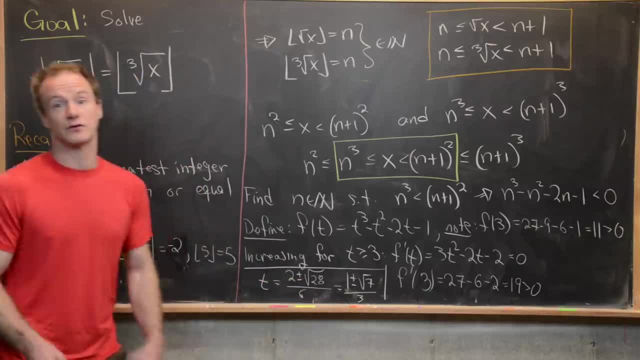 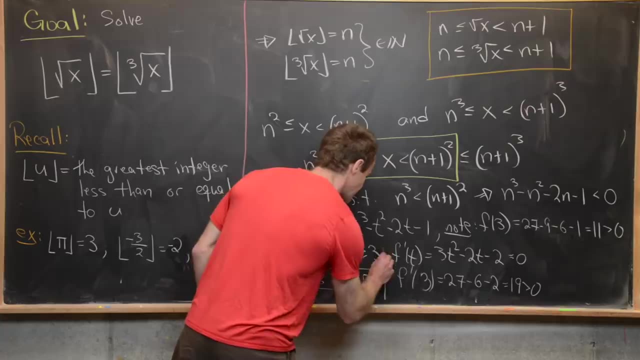 So that means it's increasing at 3.. And since 3 is to the right of the last place, that it can change from decreasing to increasing, then that means Yes, we have just checked that- it's always increasing for t bigger than or equal to 3.. 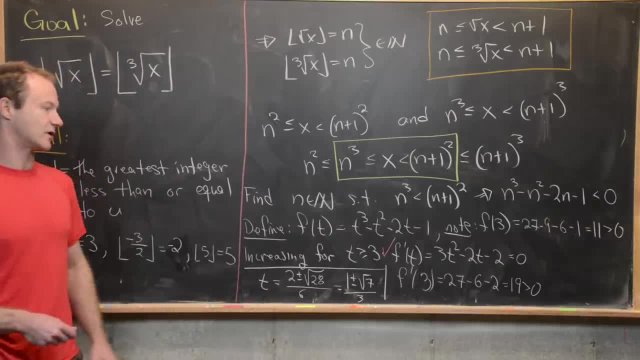 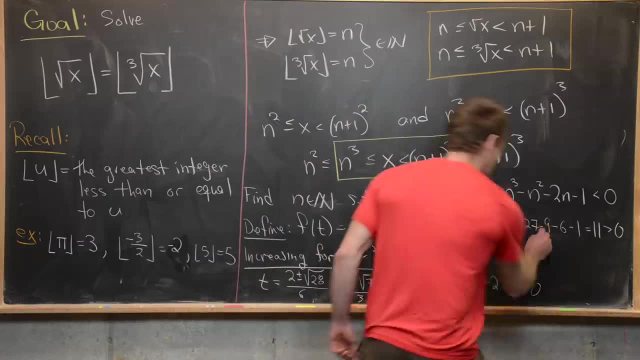 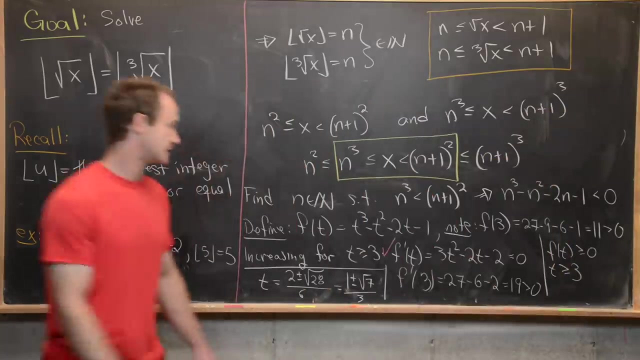 But then the fact that it's increasing everywhere after t equals 3 and it's positive at t equals 3, then that tells us that f of t is bigger than or equal to 0, for t bigger than or equal to 3.. Great. 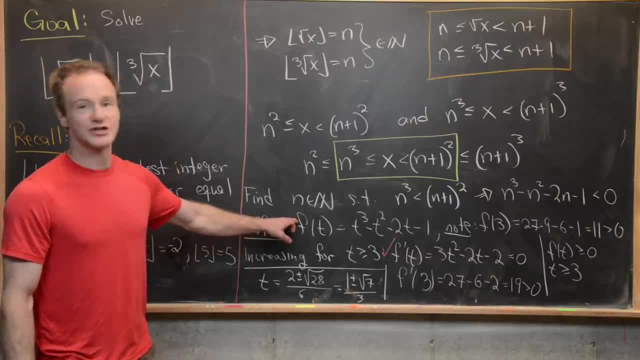 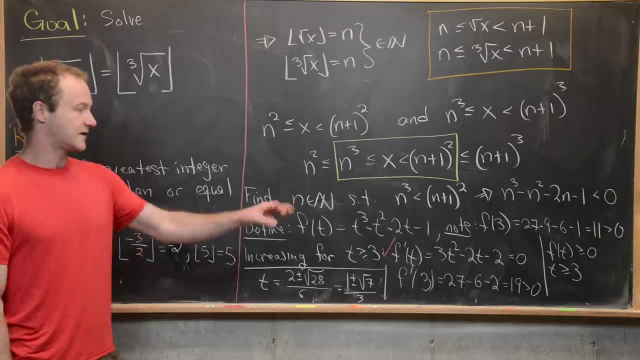 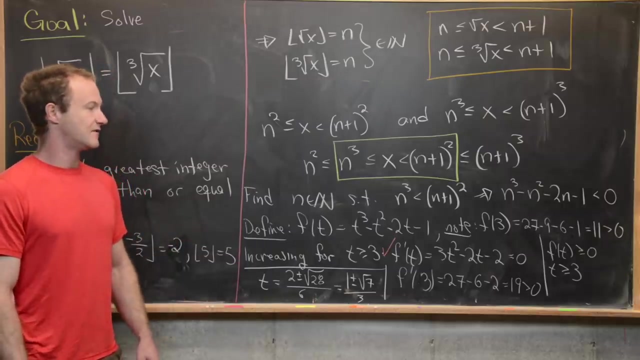 So let's see what we've got here. We've got this function, Okay. So this is like a continuous version of the left-hand side of this. inequality is bigger than 0 if t is bigger than or equal to 3, which means this inequality does not hold. 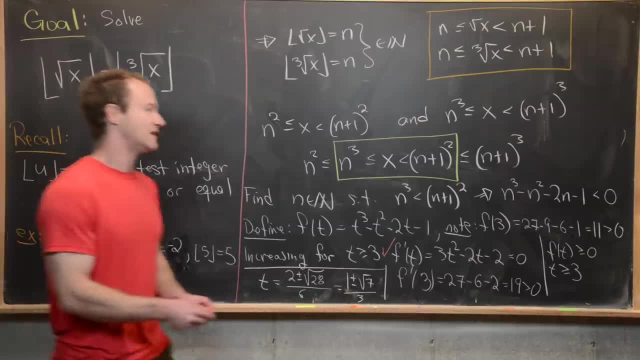 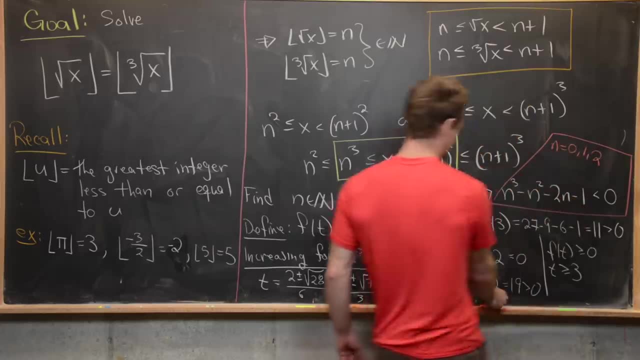 if n is bigger than or equal to 3.. But that tells us that this is only going to hold for n equals 0,, 1, or 2.. If you have any n value larger than that, then you have to stop. 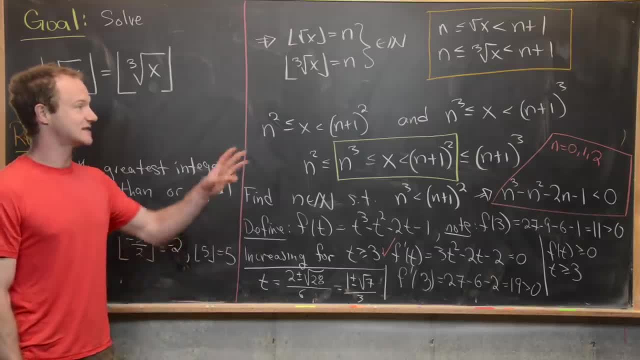 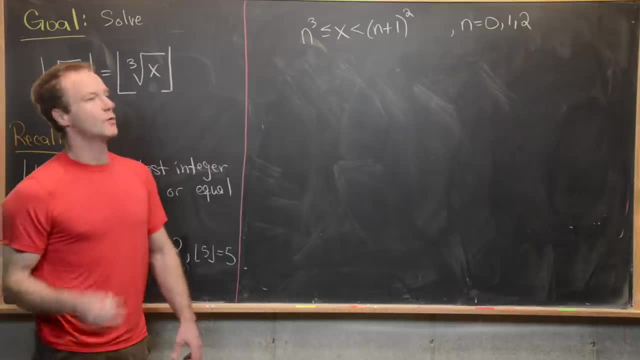 You're not good to go. So that means we really just need to check cases here, for n equals 0,, 1, and 2.. So let's maybe clean this up and we'll do just that. So on the last board we used some arguments involving just basic algebra and then calculus. 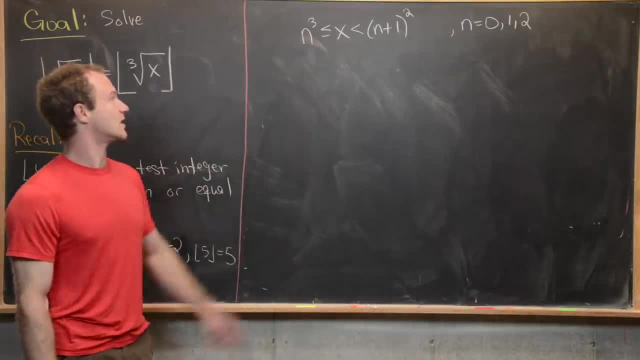 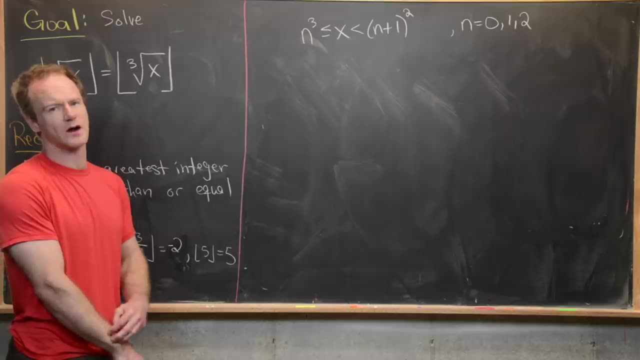 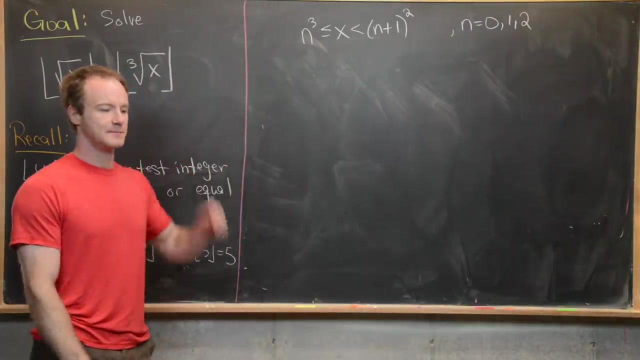 1 to show that we really wanted this inequality here, where x is bigger than or equal to n cubed and less than n plus 1 squared. So those are the types of values of x. Okay, Let's make this floor equation satisfied. 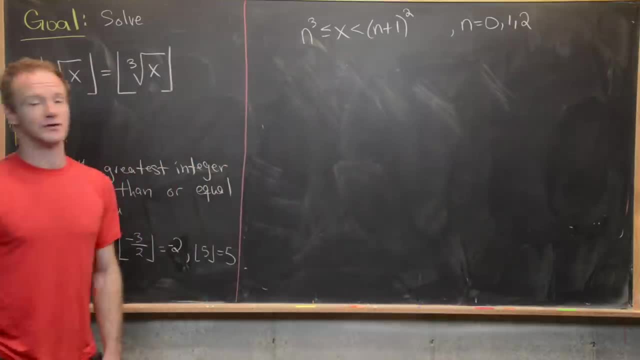 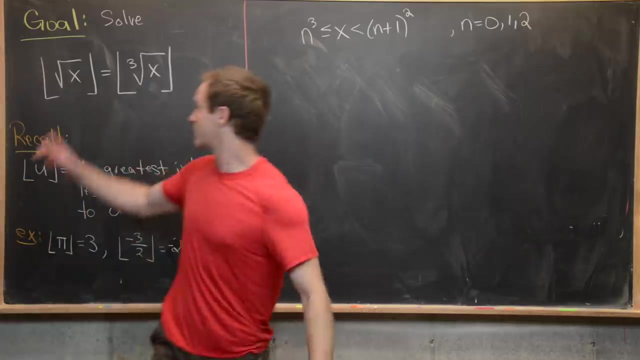 Then we also showed that the only possible n values here, in other words the only possible non-negative integer values here, were n equals 0,, 1, or 2.. And you might say: well, what about negative integers? Well, negative integers will not play into this, because we've got the square root of 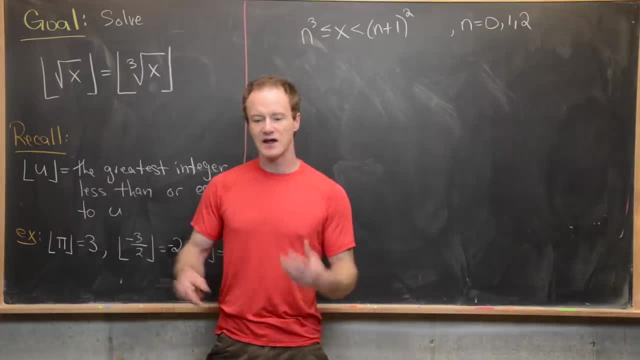 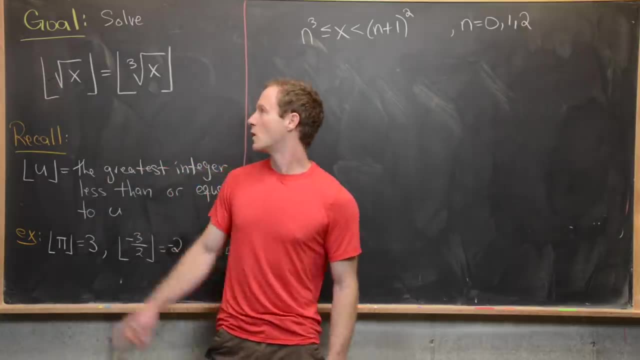 x over here, which is always non-negative. Now I think it's maybe an interesting companion question to answer this, Maybe when we had a minus sign in front here, or maybe you've got two different odd roots on either side of the equation, but I'll let you guys think about that. 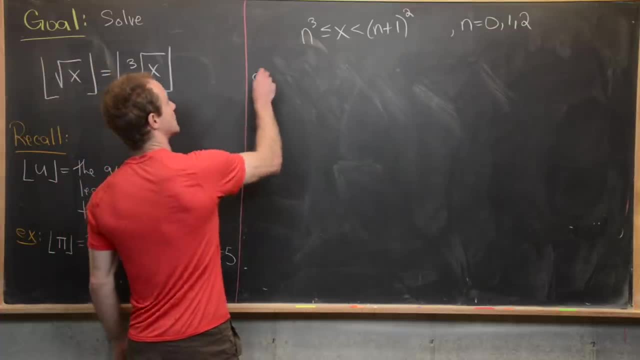 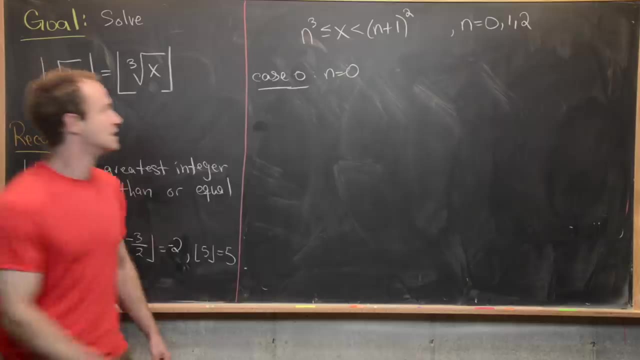 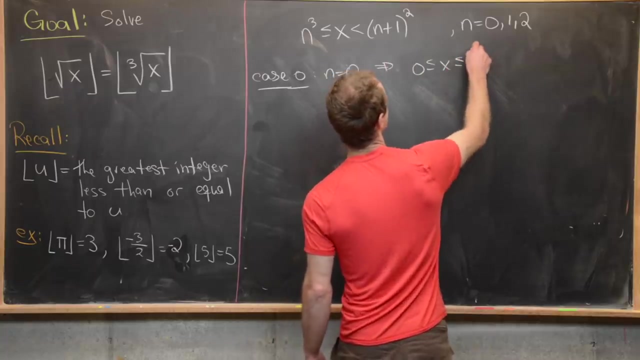 So now we just need to do these three cases. So case number one, or actually let's maybe say case number zero, which will be n equals 0. So if n equals 0, that tells us that x is between 0 and 1 squared. 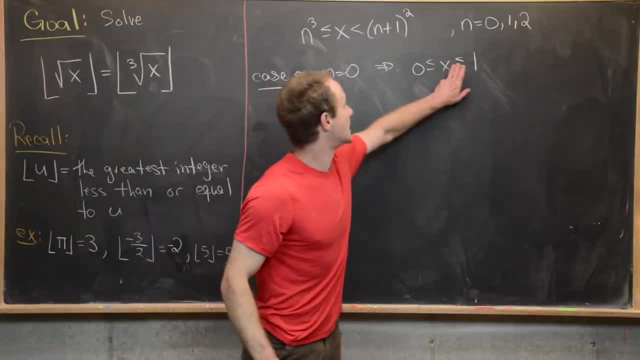 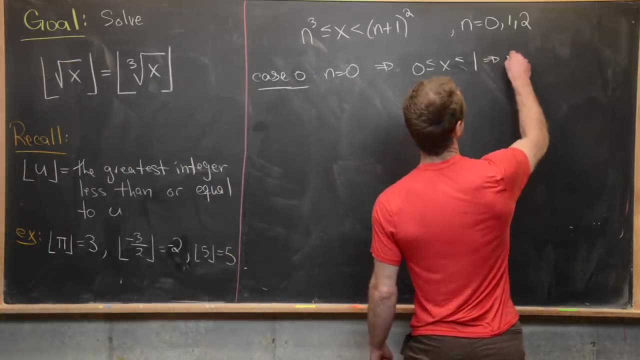 So in other words, x is between 0 and 1.. Okay, Okay, So x is between 0 and 1, not including 1.. Good, So next, maybe we could put this into a half open interval, So that means x is on the half open interval 0 to 1, including 0,, not including 1.. 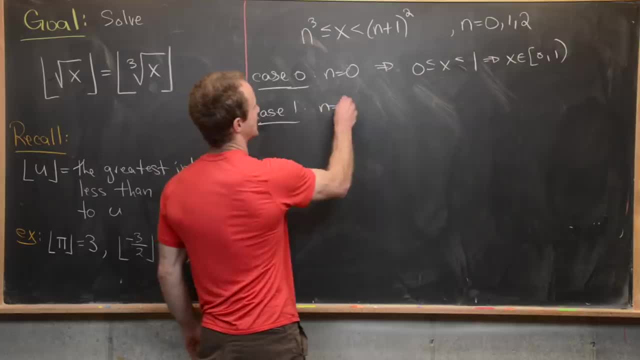 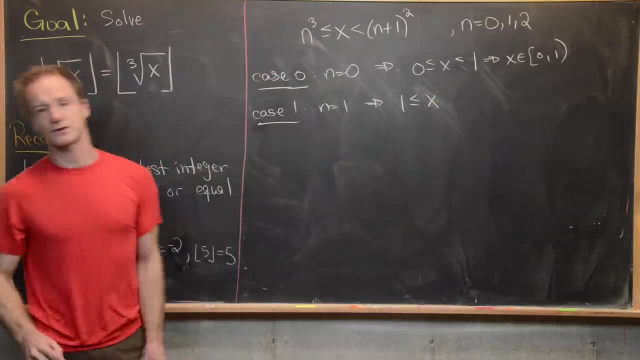 So now maybe case number one would be: n equals 1, but that tells us that x is between 1 and then 1 plus 1 squared, but that's going to be 4.. But then we can make that a half open interval as well. 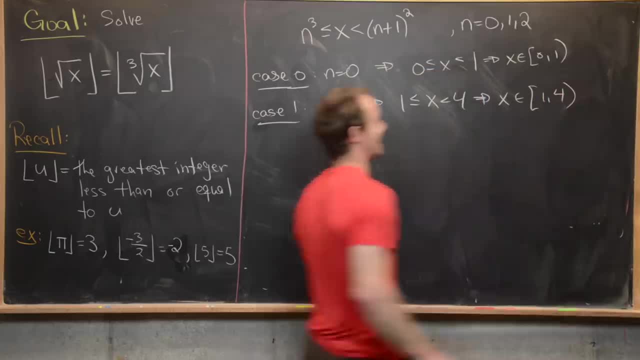 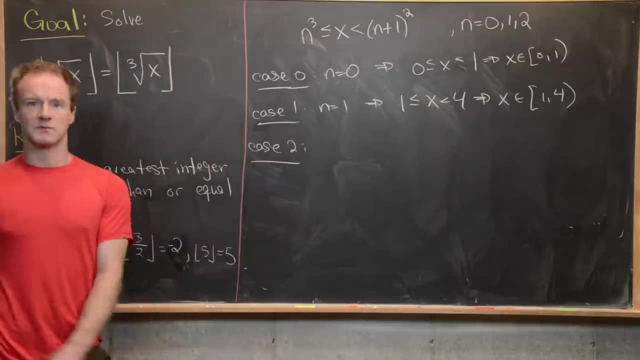 So that's going to be the half open interval 1 to 4, not including 4.. Then, finally, we'll have our third case, case two. I'm counting like a computer scientist, So we've got n equals 2.. 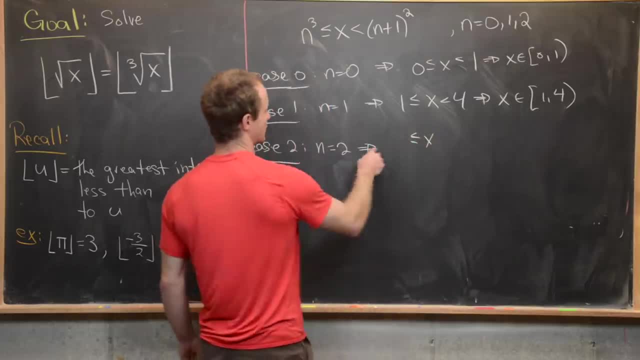 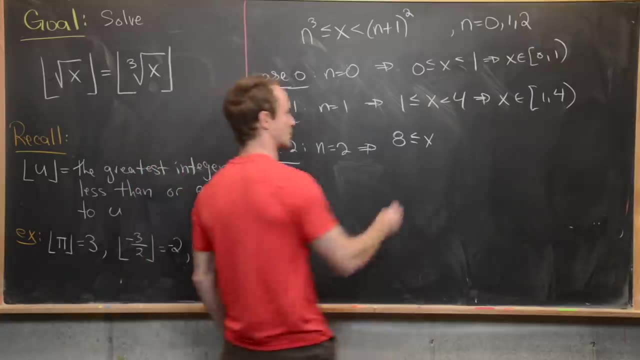 So that means we've got x is going to be bigger than or equal to 2 cubed, which is 8.. But it's going to be less than 2 plus 1 squared, Okay. Okay. So that's 3 squared, which is 9.. 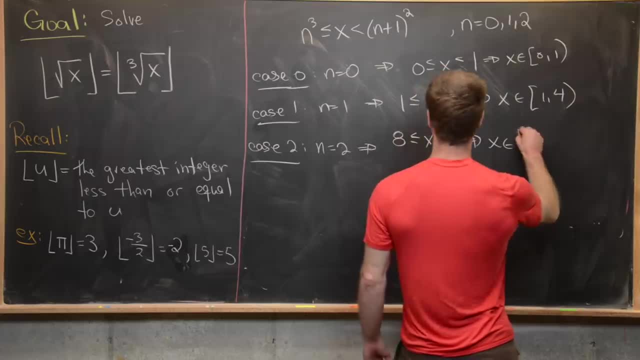 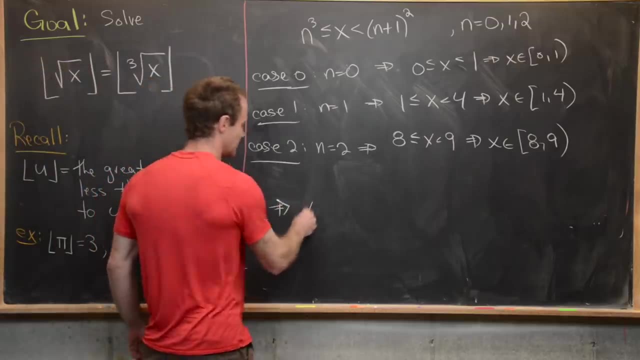 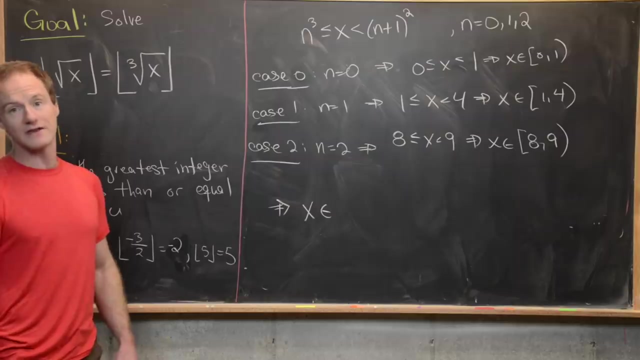 But that tells us that x is on the half open interval 8 to 9, not including 9.. So in the end we get: x is on the union of these three intervals, because either of the or any of these three cases is possible. 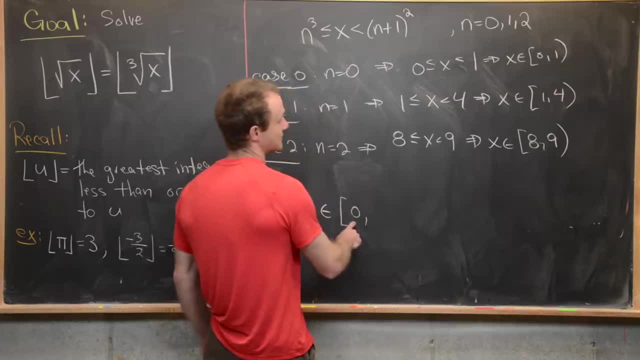 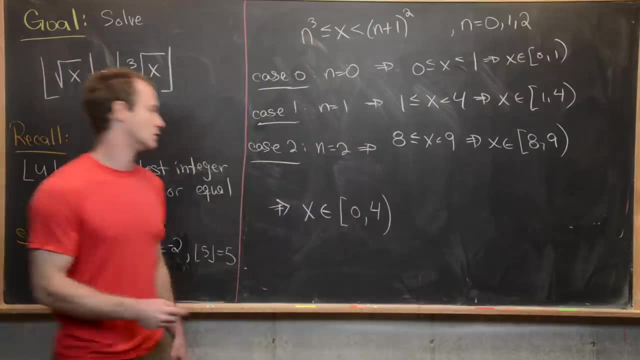 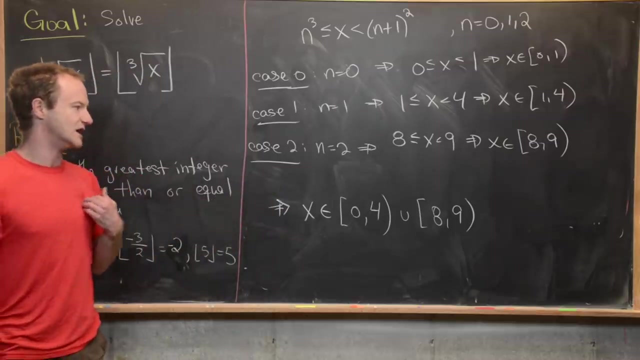 So that means we've got x is in the interval from 0 to 4.. Notice that if we union those two intervals together we just get the interval from 0 to 4.. So that's kind of cool. Union this interval 8 to 9, where we include 0 and 8, but we do not include 4 and 9.. 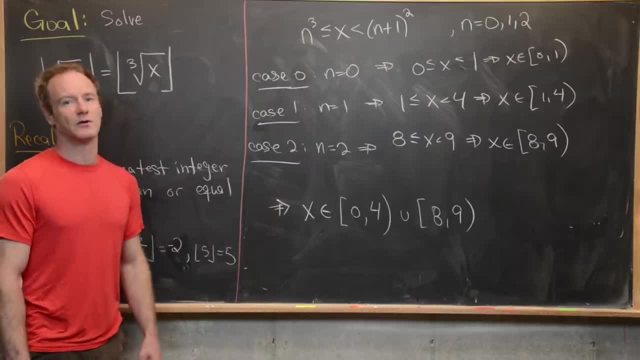 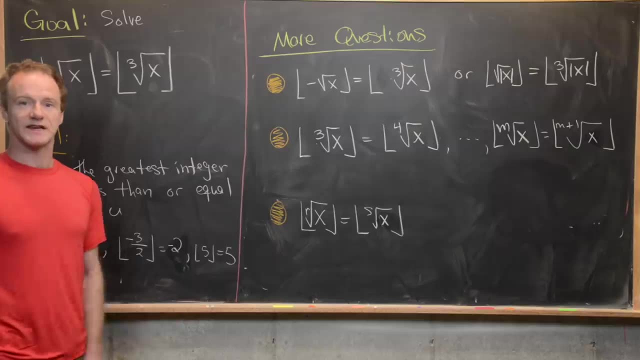 So I'll go ahead and clean this up, but I want to give you guys some followup questions that you can maybe try that are similar to this. So, looking at that problem, I think there are some obvious generalizations that are also interesting. 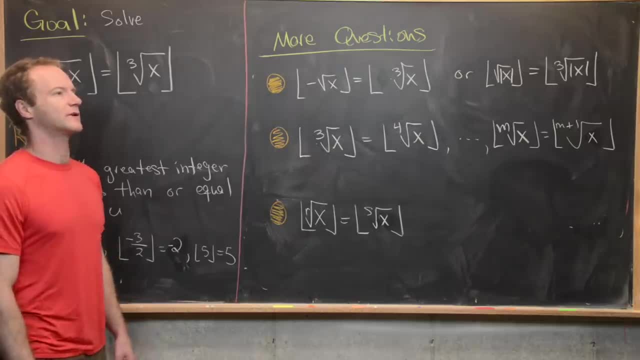 So maybe this first one involves some that are quite simple, probably fall to the same strategies that we saw in our equation. That would be: maybe the floor of negative, the square root of x, equals the floor of the cube root of x, Maybe with or without a minus sign in there. I. 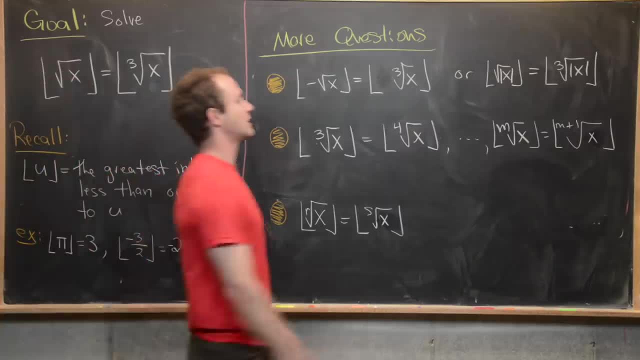 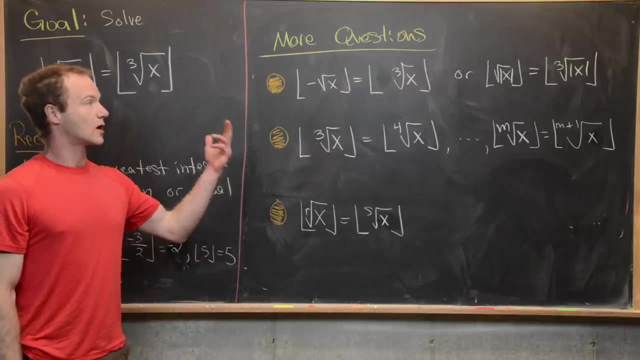 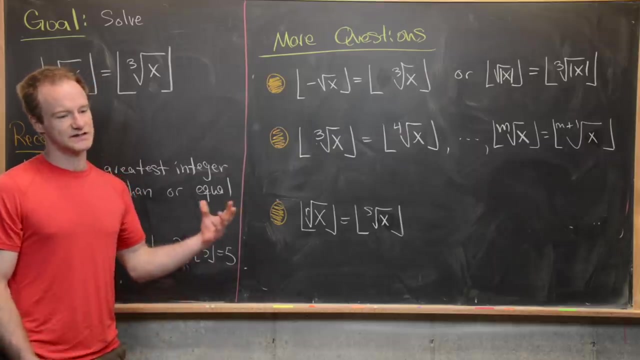 think both of those would be interesting. Or we could look at: the floor of the square root of that absolute value of x equals the floor of the cube root of the absolute value of x. So I think that one's interesting because that's going to allow all integers instead of just like positive integers. 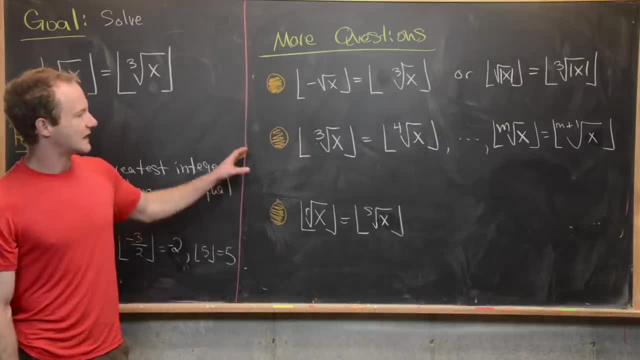 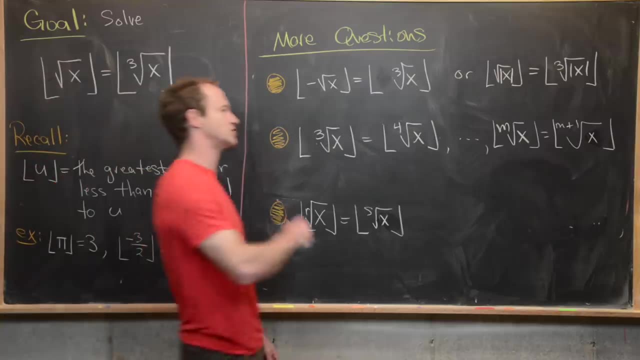 to enter the argument at that stage. And then here are some others. Maybe we could say: well, what about when is the floor of the cube root of x equal to the floor of the fourth root of x? Or, more generally, when is the floor of the nth root of x equal to the floor of the m plus first root of x? 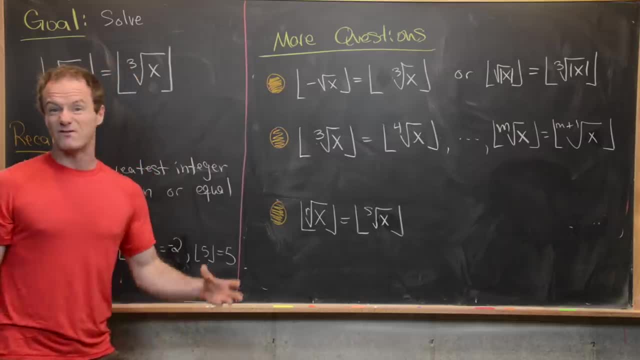 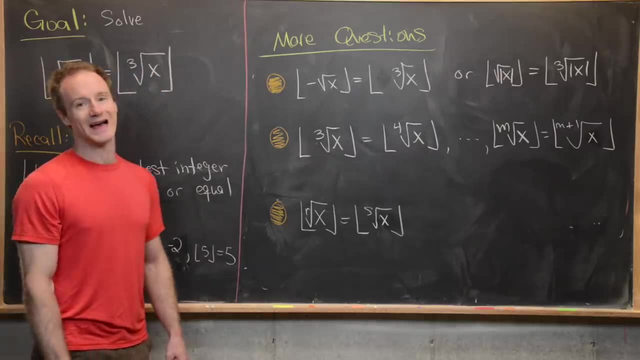 And then super generally is: let's say we fix r and s arbitrarily. When is the floor of the nth root of x equal to the floor of the m plus first root of x? When is the floor of the rth root of x equal to the floor of the sth root of x? So maybe go ahead. 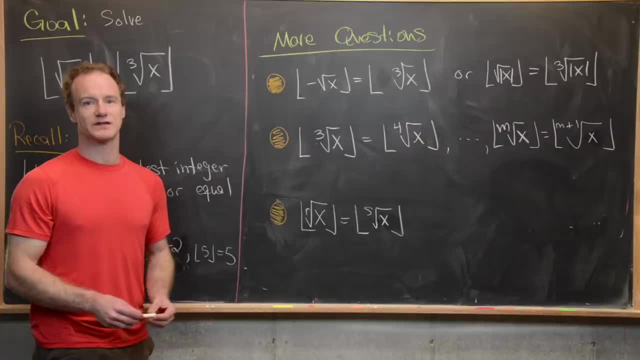 and play around with these and post what you get in the comments, And that's a good place to stop.